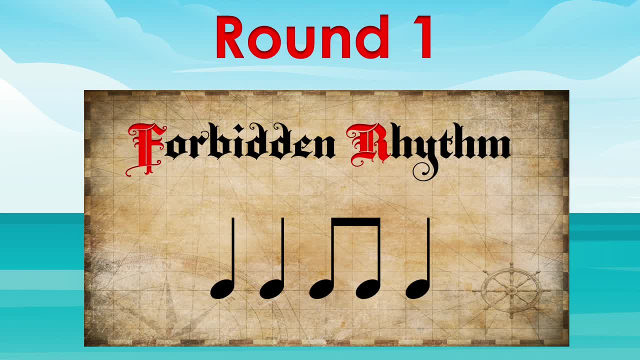 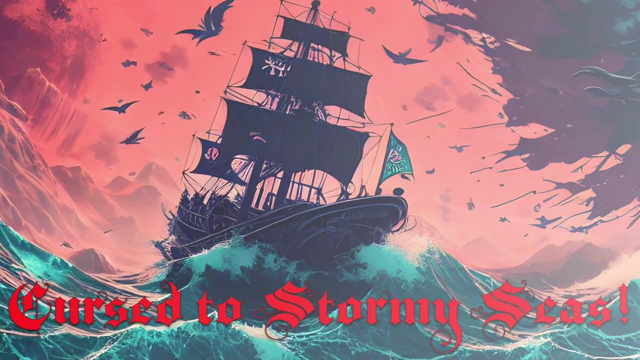 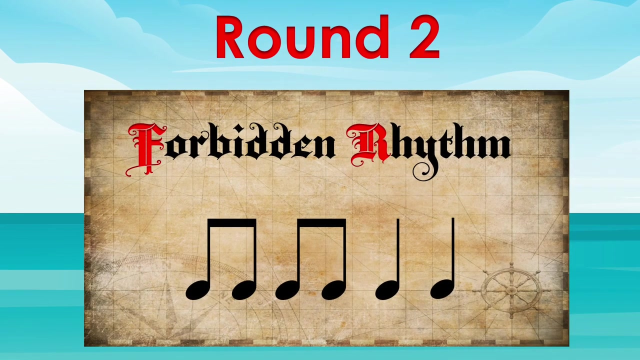 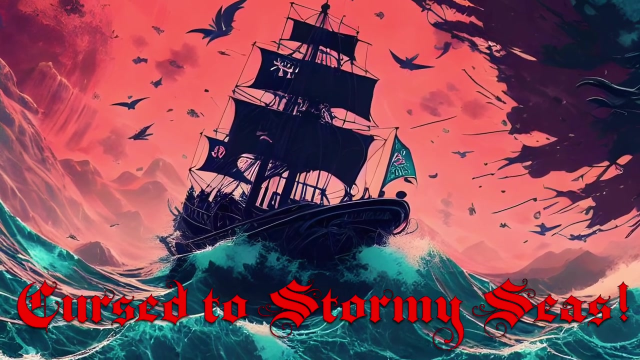 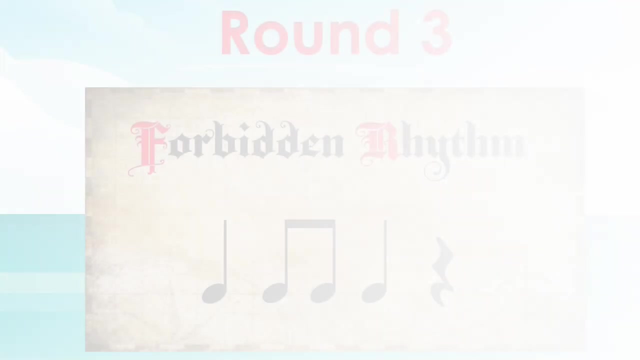 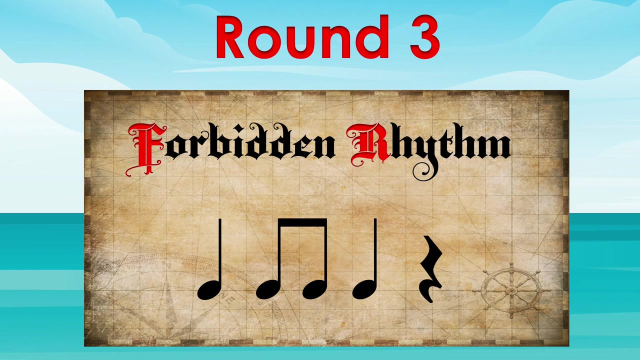 Let's go, C'mon, Let's go. great job friends. now let's try round two, a different forbidden rhythm, but the rules are the same. are you ready? let's go? so excellent job, friends. now it's time for round three. we are adding some extra things, like a rest. 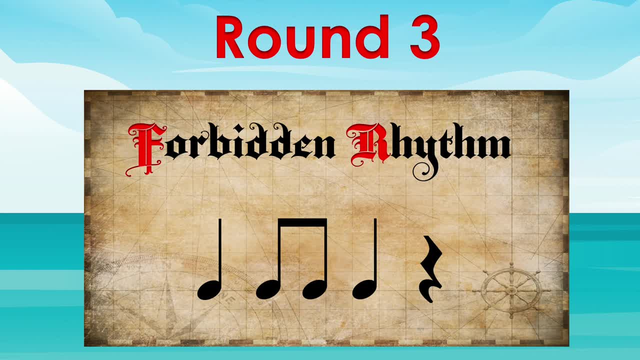